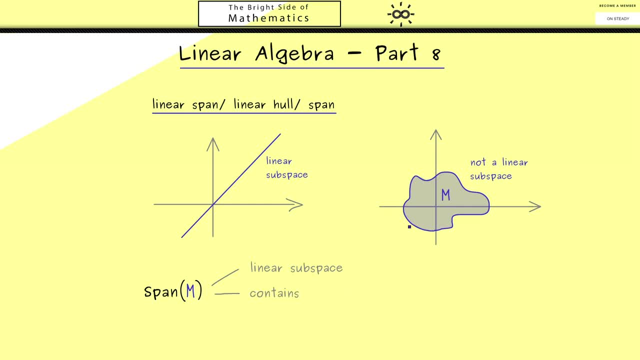 it contains the set m, ZM, but then it also contains all possible linear combinations of vectors of M. Of course this is needed because otherwise it wouldn't be a linear subspace, And, lastly, we want to define it as the smallest subspace with this. 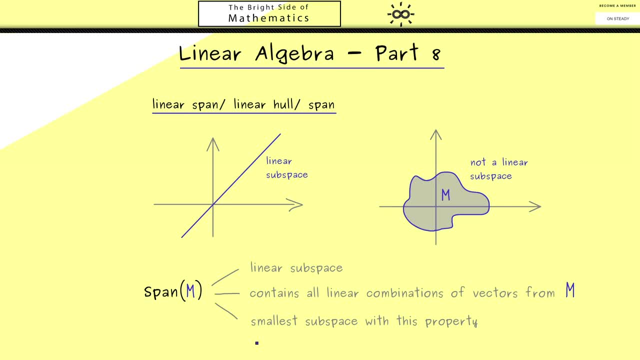 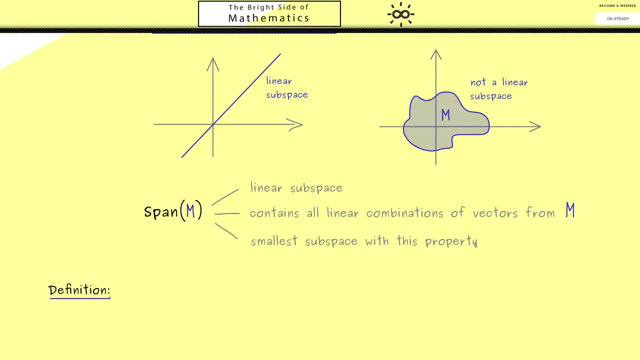 property, And smallest here simply means with respect to the subset relation of sets. Therefore, span is already well defined with these properties here, However, maybe let's put this into a more concrete definition. So here what we need is a non-empty set M which consists of vectors in Rn- You see how many. 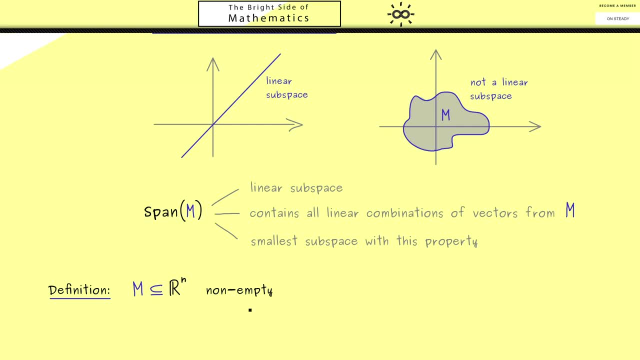 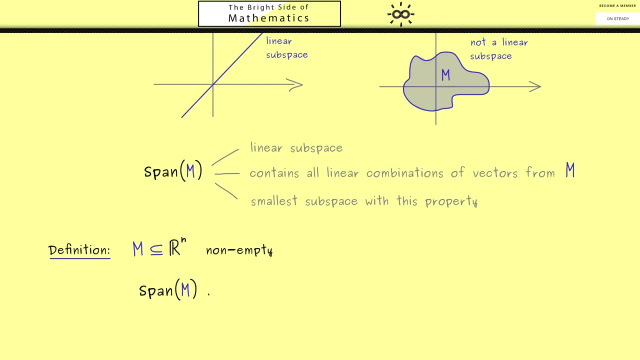 elements. the set M has is not important, but we need at least one. And then we can define a new set we call span. So we can define a new set we call span. So we can define a new set we call span, Which by definition consists of vectors in Rn as well, More precisely, each. 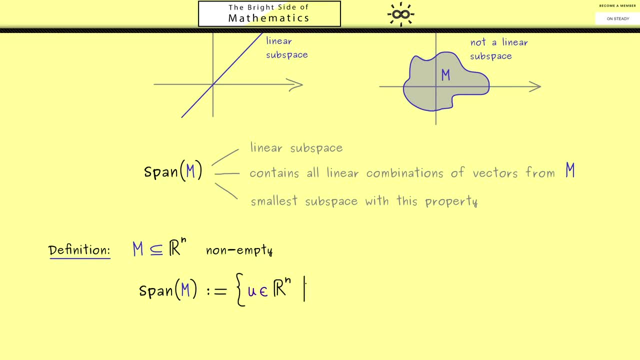 vector u in this set should be given by a linear combination. Hence what we need are scalars lambda j in R and vectors uj. However, the important part here is the vectors uj come from the set M, And then we can write our vector u as a sum over. 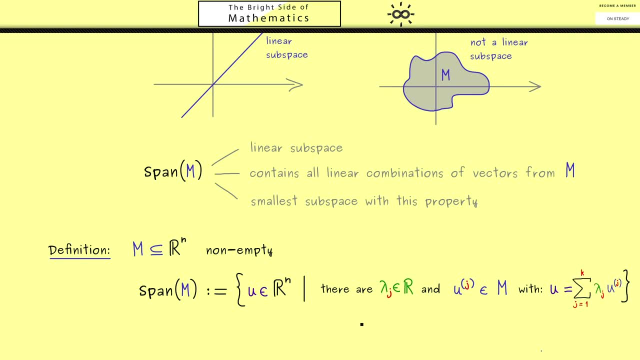 lambda, j and uj. And there we have it. This is the precise definition of span. However, now you could ask what is about the case that M is the empty set There? we also want to give a useful definition. This means that also in this case, the span should represent a linear subspace, And 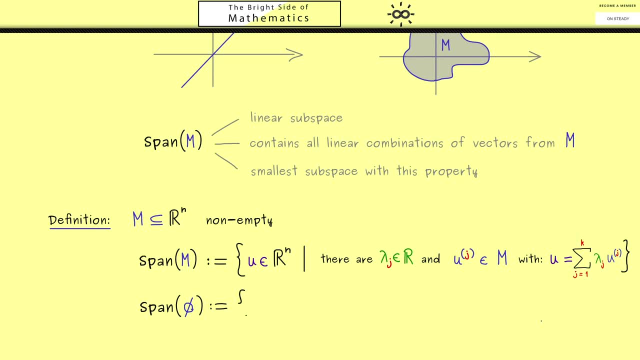 for the empty set, this should be the smallest possible one, which means we have the zero space, Which is the space that only has one element, namely the zero space, The zero vector in Rn. Ok, by having this definition, we now can look at some examples. 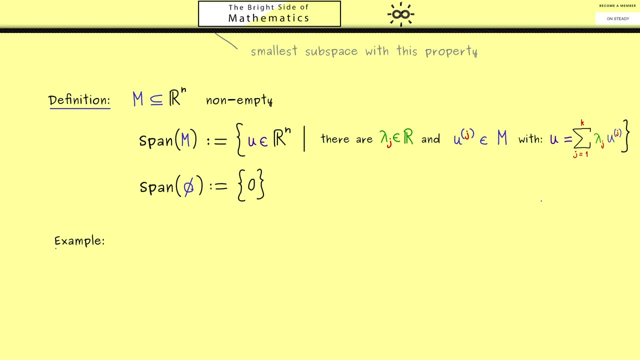 of spans. As always, let us start with an example in R2.. So maybe lets consider the set M. that only consists of one vector, namely. Of course, this is a well defined subset of R2. And, as always, we can visualize this very nicely in the plane. So here we have. 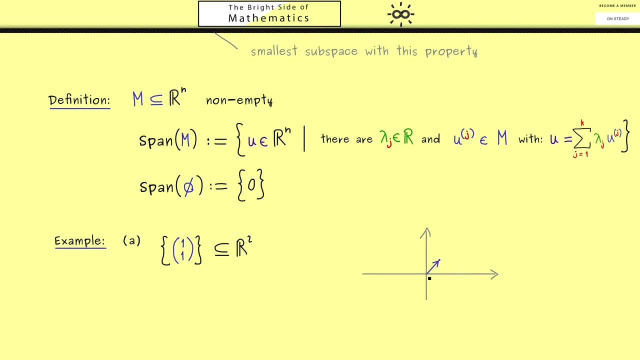 the vector. So now, by definition, the span of this set should be given by all linear combinations of this one single vector. This means that if we write it as such a set, we only need one scalar lambda, And then u should be given by lambda times, So you: 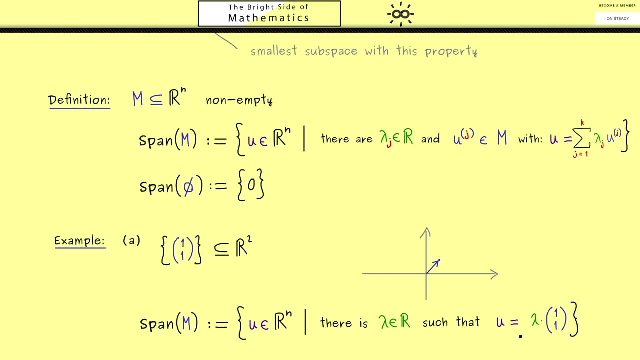 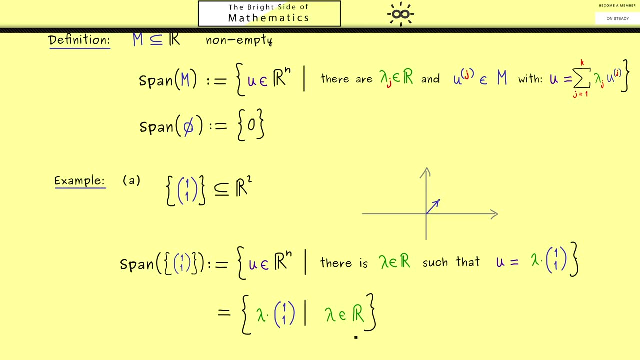 see this set looks very simple And indeed we can write it in a shorter way. One simply writes lambda times, Where lambda goes through the whole real number line. Moreover, i can also tell you now there is even a shorter notation some people use In this case. they write the set R times, the 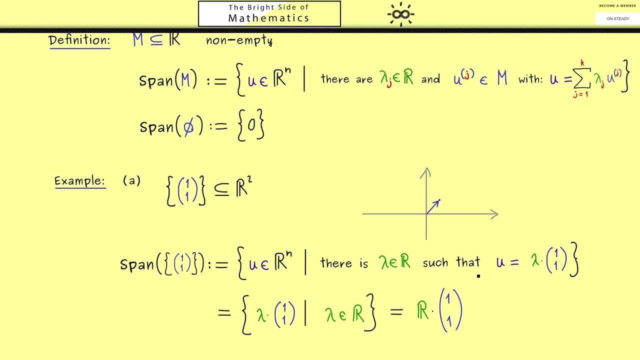 vector, And there you immediately should see this is just a short cut for the left hand side here. However, now, no matter which notation you use here, you should recognize that we already discussed such a set in part 4.. It's simply a line through the origin in the direction of: So indeed it's a subspace. 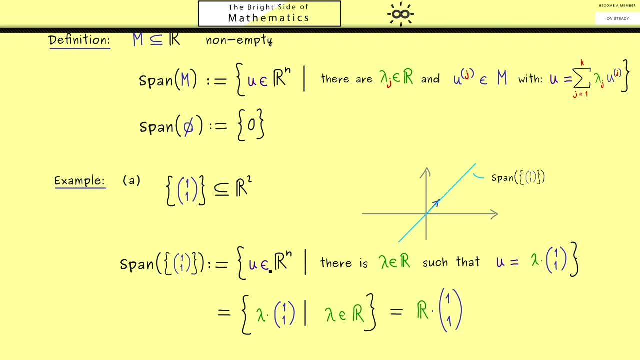 that contains our single vector. Ok then, maybe the last notation i should tell you about is that sometimes one omits the brackets, the set brackets in the span here. In other words, one simply writes span of the vector. So you see, this notation here is. 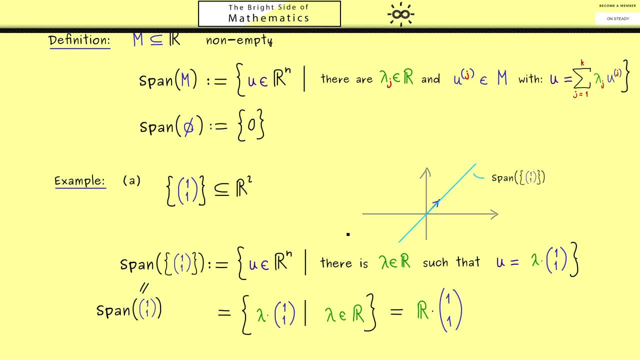 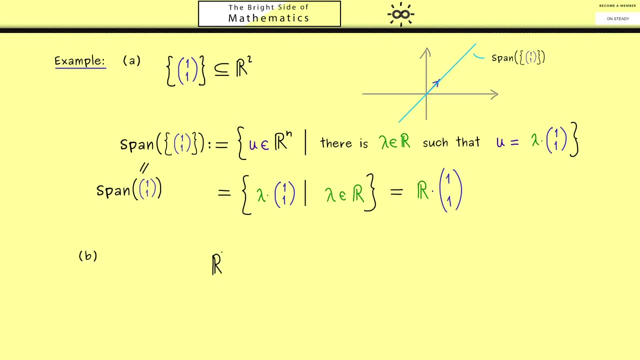 almost as short as the right hand side here. So this notation here is almost as short as the right hand side here. Ok, then with this let's go to the next example, And this one should be 1 in R3.. And then let's consider a set consisting of two vectors. 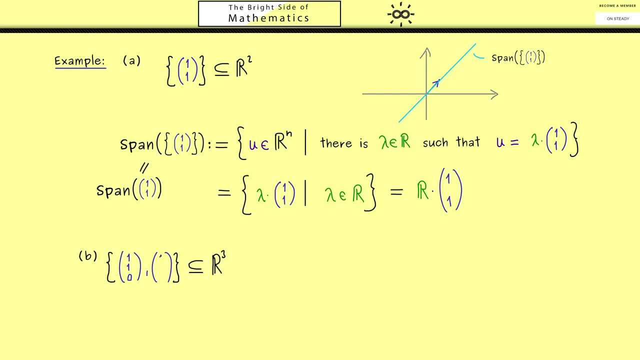 The first should be, and the second. And now the question for you is: what is the span of this set? And, as before, often one omits the set brackets, So maybe let's first try to visualize this in the space. So we have three axes where this one is the first one, this one is the second one and